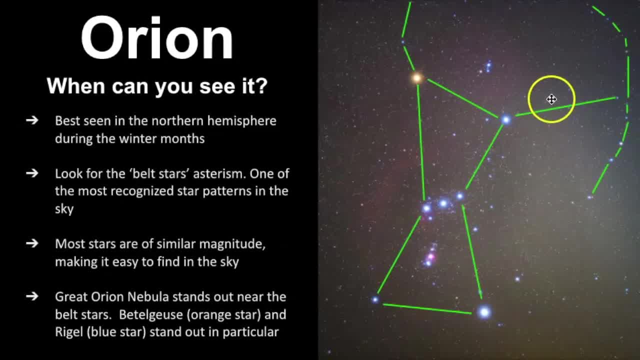 what the star pattern looks like, at least a portion of it. Most people recognize Orion as these main seven stars. What's really great about these seven stars is that they're a similar magnitude, so it really makes it easy to find in the sky. So when can you see it? Remember, here at Learn the Sky, I always 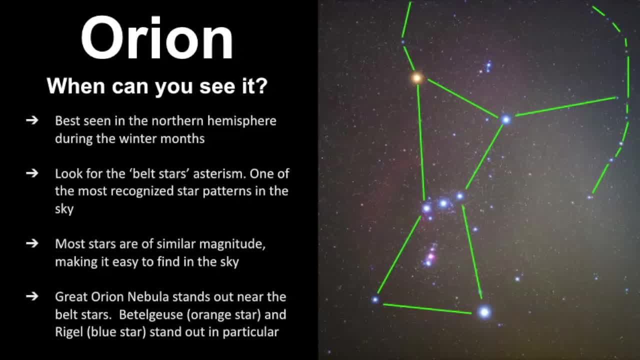 teach from the perspective of the Northern Hemisphere, because that's where I live. I have never seen Orion from the Southern Hemisphere, but for the Northern Hemisphere it's best seen in the winter months. You want to look for the belt stars, asterism- This, of course, is one of the most recognized. 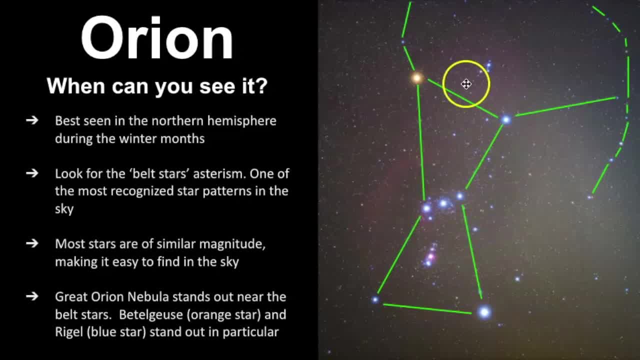 star patterns in the sky. As I said, each of these main stars are of similar magnitude I found out. a really fun fact about this constellation is that all these seven main stars are expected to become supernovae, Which is really, really cool. There are some other things that really stand out. 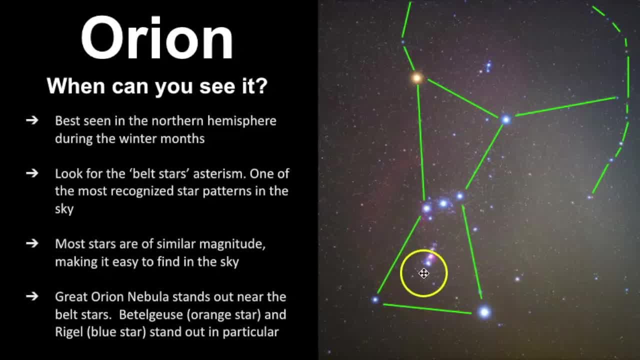 in this constellation as well. The Great Orion Nebula is right underneath those belt stars and there are some well-known stars such as Betelgeuse, or some pronounce it Betelgeuse or Betelgeuse. I was taught that it was pronounced. 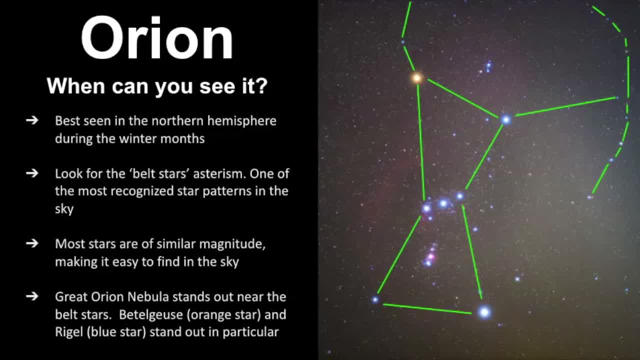 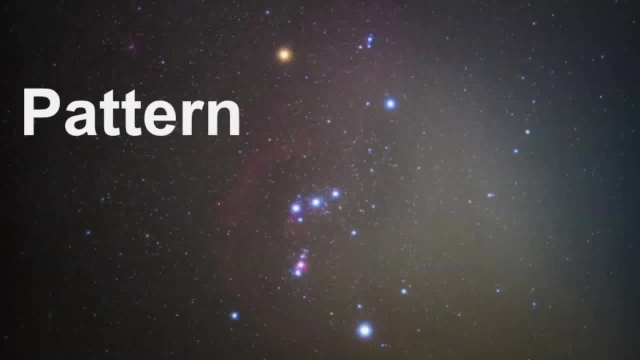 Betelgeuse, so that's the way I kind of that's my default pronunciation of it, And then also Rigel. right here is another really bright blue star. Now we'll take a look at the star pattern that Orion makes across the 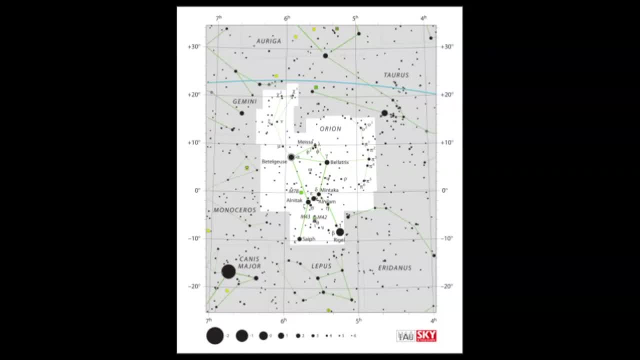 sky. Here we have the official star map of Orion released by the International Astronomical Union, and the things I want to point out to you are to show you how Orion can be a guide to everything surrounding it in the sky. So here you can see the belt stars. this is the best. 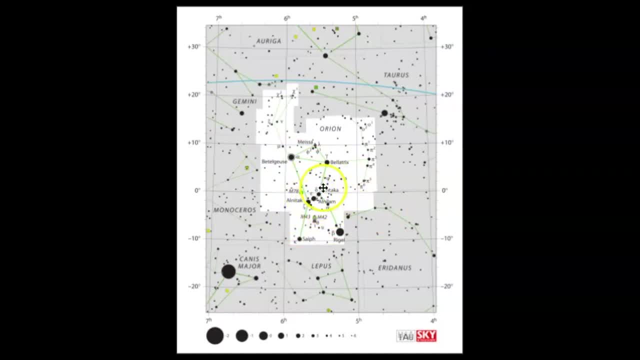 way to find Orion is to look for these three stars in a row, And you can use stars to point down to Canis Major, which is this bright star is known as Sirius, the brightest star in the night sky. And then you can also use the belt stars to 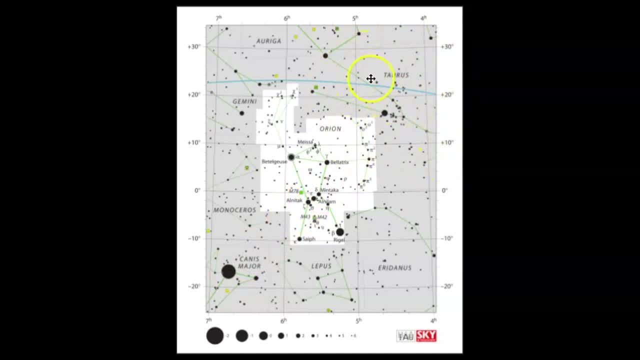 point up towards Taurus right here, which is Taurus is represented as a bull. If you want to learn more about that constellation, go see that video. Then you can use Rigel and Betelgeuse If you draw an imaginary line through those two. 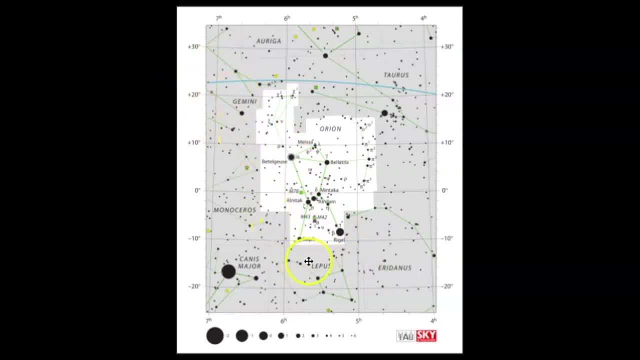 bright stars, it'll lead you to Gemini. If you do the opposite, knee and shoulder star, you have safe here. and Bellatrix, Draw an imaginary line up this direction, you will find Auriga. You can also use the two shoulder stars to guide you. 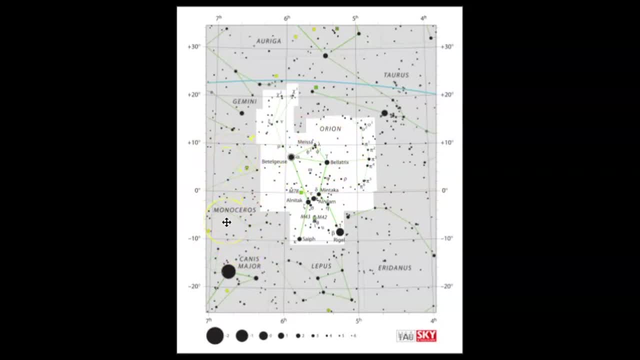 towards Monoceros, which is known as the unicorn, a super faint constellation. I've got a video on that. Be sure to see more about that video in the links posted below. But you can also use the shoulder stars if you go past Monoceros over in. 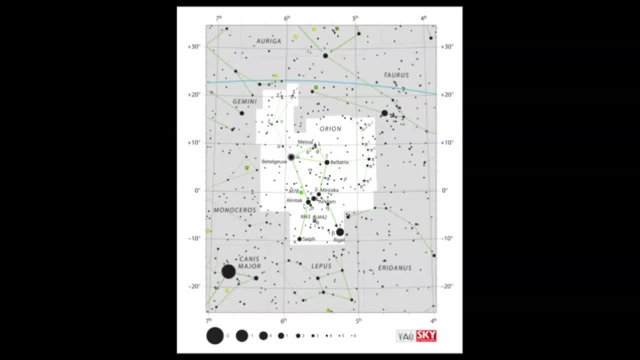 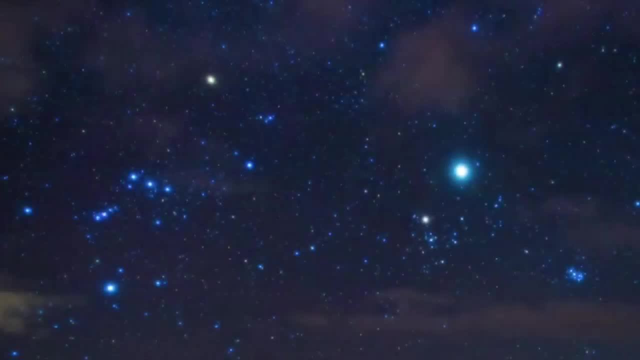 this direction is where you would find Canis Minor. So if you can find Orion in the sky, you can find everything else. So let's get some practice with how to find Orion. So first, we've seen this picture before. Here is where Orion is. You can see the belt stars, You can see the Sword of 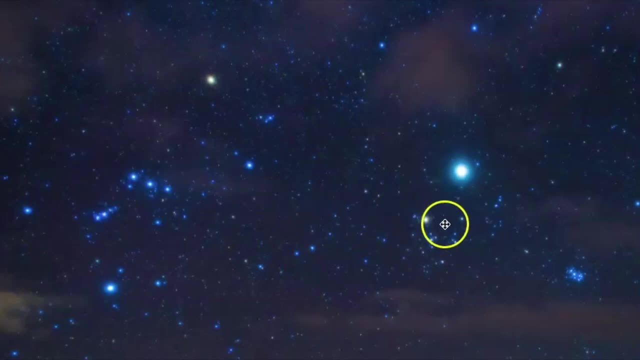 Orion, and you use the belt stars to point towards Aldebaran, which is the bright star, and Taurus. Here's the v-shaped face of Taurus, And then here's the Pleiades. This is a planet that is traveling through Taurus because of 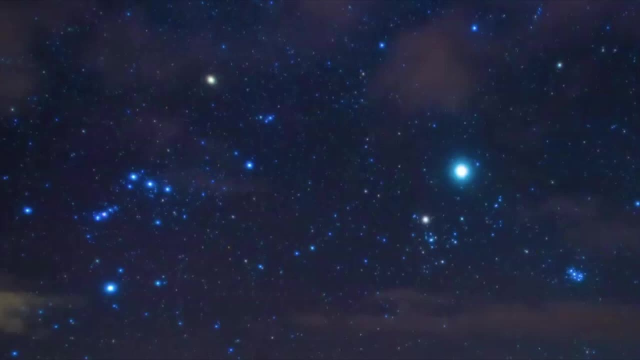 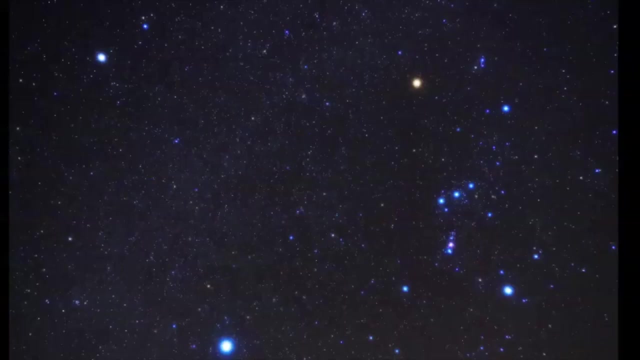 it is a zodiacal constellation. So remember, zodiacal constellations are ones in which the sun, moon and stars pass through. Let's get another view of Taurus because, remember, the more pictures you see, the better you can get at identifying these constellations, And in this one you can. 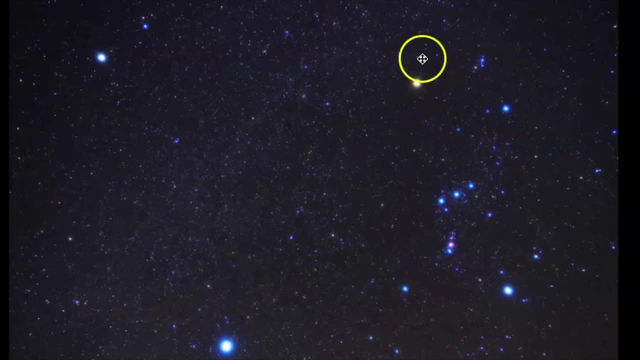 see also another familiar star pattern known as the winter triangle. The winter triangle is not a constellation but an asterism And an asterism I've got a whole video on that, so be sure to go see that video. but an asterism is really another shape or pattern either within a constellation. 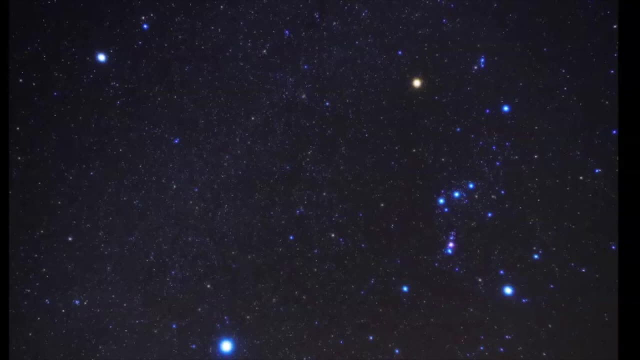 or made up of bright stars, of constellations, and you can use it to find other constellations in the sky. So here we have Orion, down here is Sirius, that's the bright star in the constellation known as Canis Major, And then here is Procyon, or Procyon- I've heard it pronounced both ways- And this two. 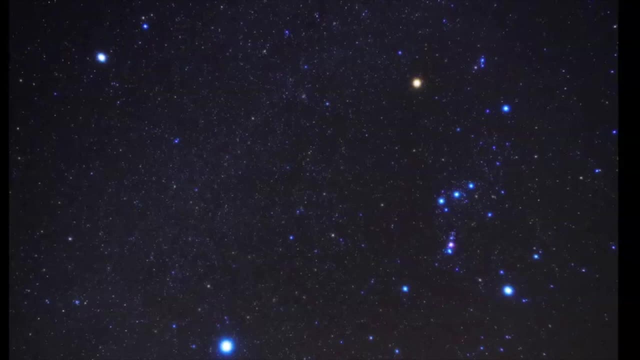 this small two-star constellation is known as Canis Minor, And these are the hunting dogs of Orion. So again, if we were to use Orion as a guide to the sky, this is what I teach all of my students: you can use the shoulders to point to Canis Minor. you can use the belt to point to 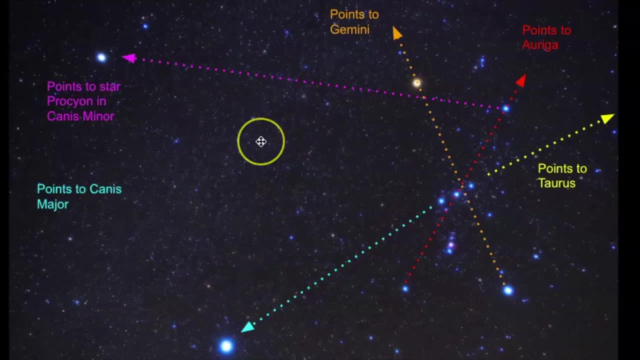 Canis. Major Right in this arena is Monoceros, a unicorn constellation, a modern day constellation, And then here, if you use these two stars to point to Gemini, this points to Auriga and then this points to Taurus. So I will say it again: 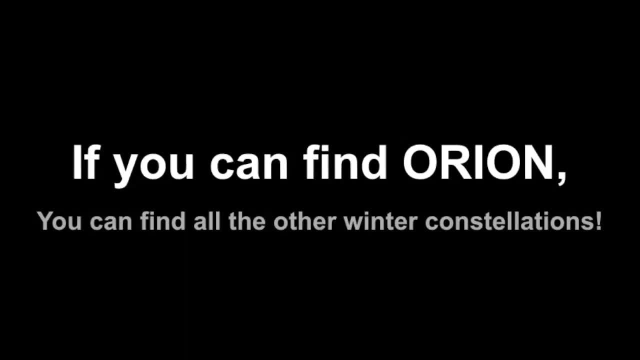 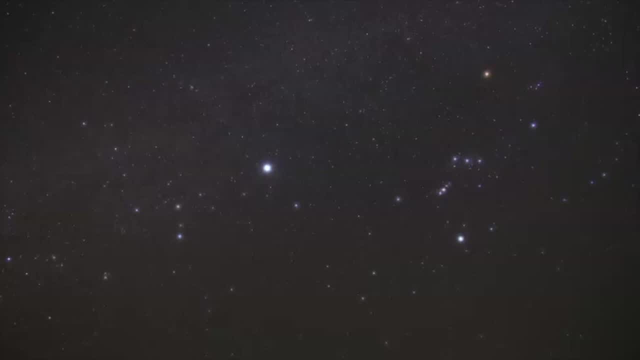 if you can find Orion, you can find all the other winter constellations in the northern hemisphere. I've got a few more pictures for us to review, because of course, practice makes perfect, Perfect, Perfect. So here we have Orion and we have Canis, Major, Orion's hunting dog. There's also another constellation called 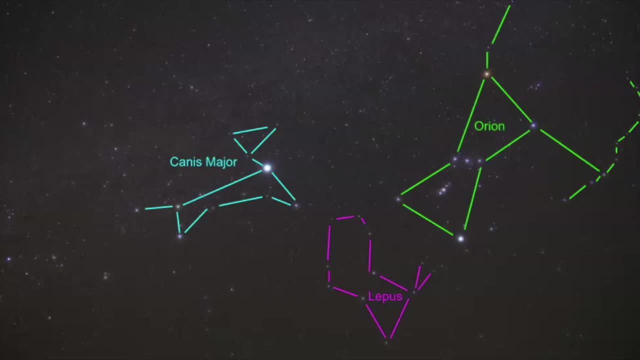 Lepus, the hare, And if we were to point these out, here is where they are. So we've got Orion right here. Here is Lepus, This is known as the hare, And then we have Canis Major. here You can also see some of the Milky Way. 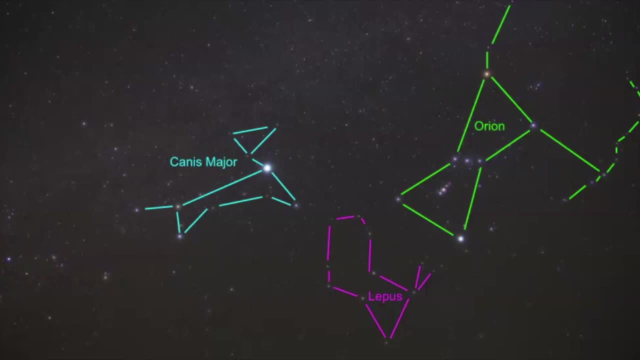 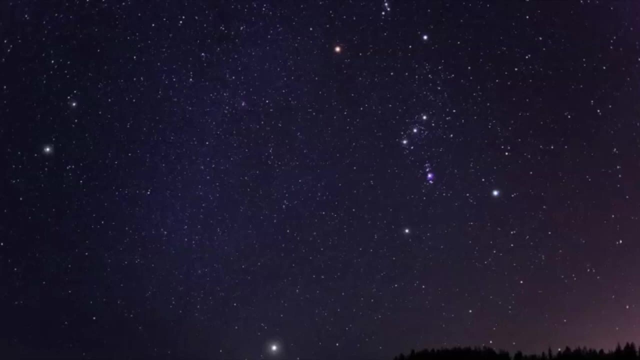 right here. It's pretty faint in the background, but it is there. And then is that constellation that I have no shortage of pictures, So as we go through, you should be able to see in this picture. you should see Orion, you should see Canis Minor. 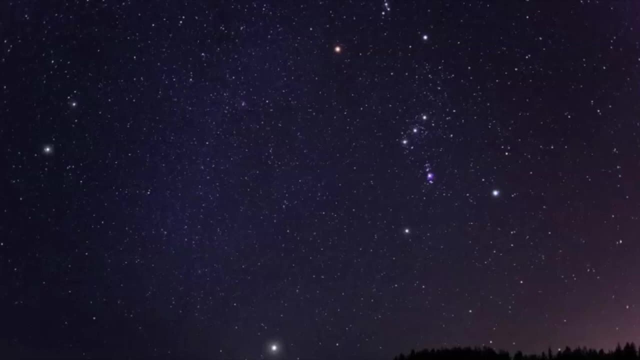 and then you should see a portion of Canis Major, but really only that bright star, And can you see that winter asterism triangle, Or winter triangle asterism, I should say? If we were to keep going, I've got more pictures. This is another gorgeous photo because 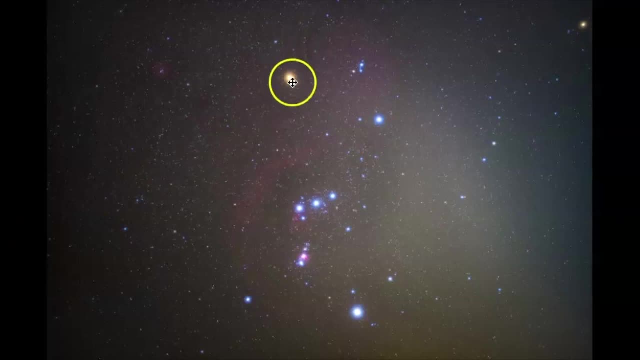 what really shines through is the color of the stars, which most of the main stars are blue, but Betelgeuse is an orangish colored star, And you can also see some of the celestial objects that are shining through in this long exposure photograph as well. 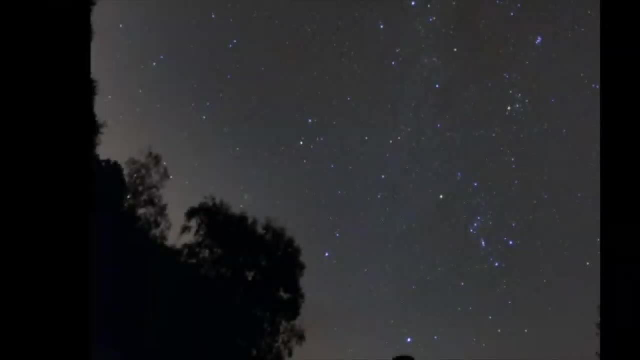 Now, Orion is not only a part of the asterism known as the winter triangle, but there's also another asterism it's a part of called the winter hexagon, And if you connect some of the brightest stars in the winter sky it makes these different star patterns. So here we have all the different constellations that 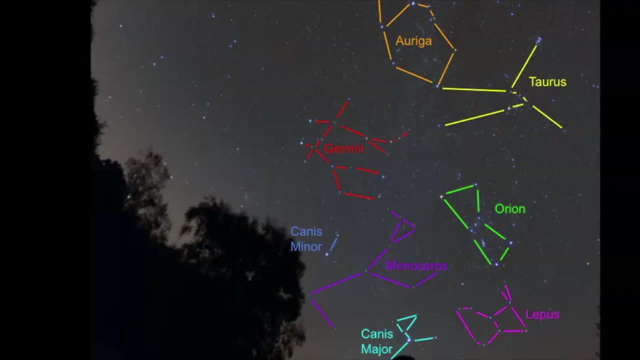 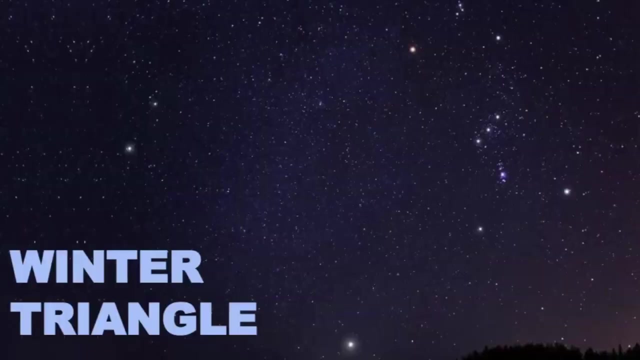 are within the winter sky And you can see there's a lot here. We've got Taurus, Auriga, Gemini, Canis Minor, Monoceros- a super faint constellation- Canis Major and Lepus. So the winter triangle, remember, is a useful asterism that connects these three. 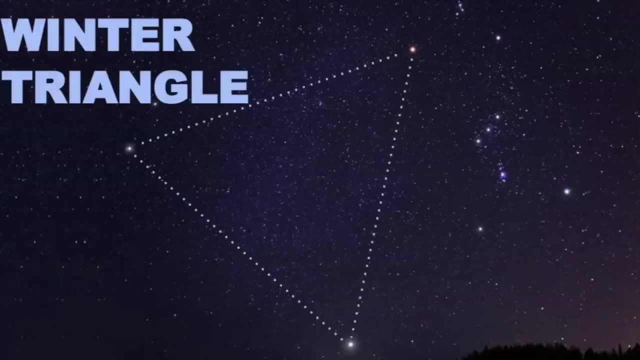 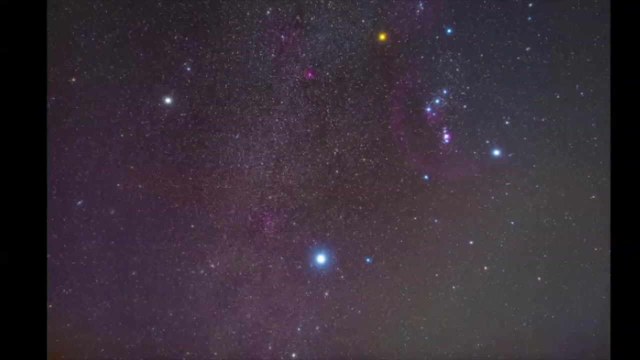 constellations in the mission And it also통 with the winter relation. I've not done a full Archaeological Deadline in here, but you can see everything in this picture here. If you're that suitable, you'll want to enter a program on AA for our logo page. Then you'll be able to have all the most because you can type in A4 here if you want to. But this: 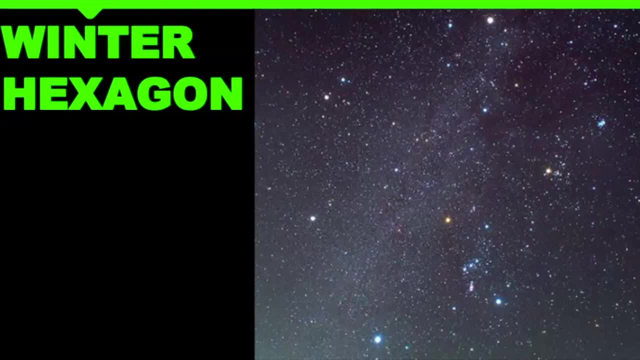 the other constellations that have very bright stars And it's a very large asterism, So it can actually be challenging to point out because it is so large in the sky. Oftentimes when I'm stargazing, there's either a mountain in the way or I'm surrounded by a rim of trees. So if you 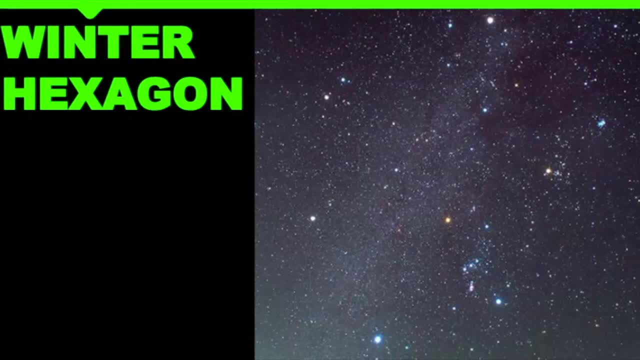 want to find the winter hexagon. you want to find like a wide open field to observe this in. And if we were to point out the winter hexagon, this is where it is located And it connects all the brightest stars that can be seen in the winter sky in the northern hemisphere. The stars include: 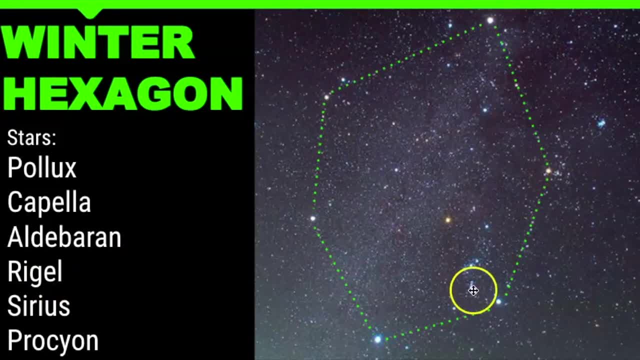 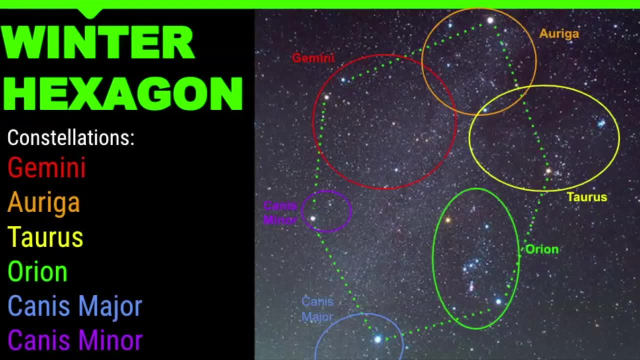 Pollux, we have Capella, we have Aldebaran, Rigel, Sirius and Procyon. And if we were to point out where all those constellations are in the sky, here is where they're located. So the winter. hexagon is a great place to point out the winter hexagon. And if we were to point out the winter hexagon, this is where it is located. And if we were to point out the winter hexagon, this is where they're located. And if we were to point out the winter hexagon, this is where they're located. And 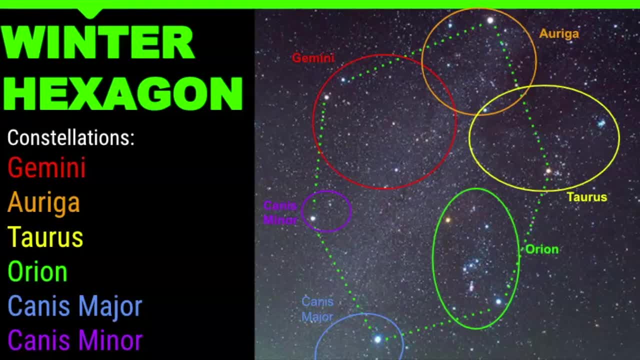 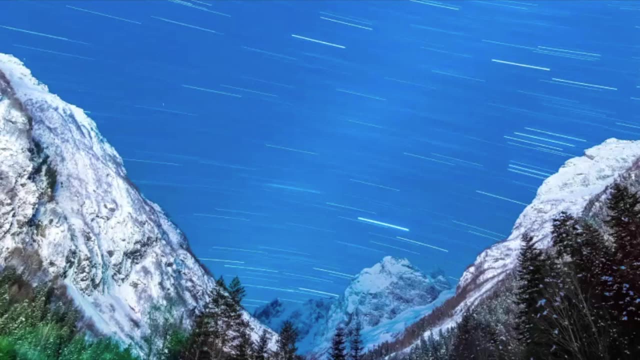 great asterism, just to help you find other constellations in the sky. And one other trick that I use to really test my students if they know where Orion is is I give them star trail pictures. So there's a few things you can see in this star trail picture. Can you find the belt? 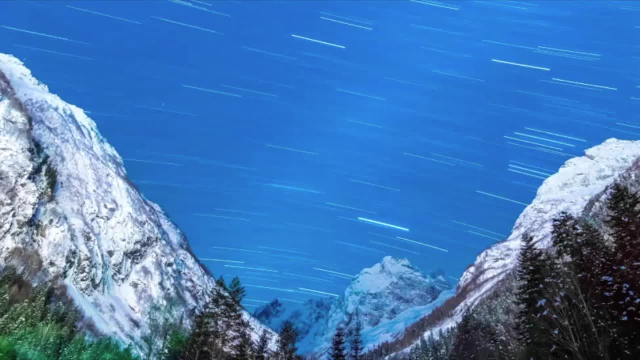 stars of Orion? Can you find the winter hexagon? Can you find Sirius, the brightest star in the sky? Can you find the belt stars of Orion? Can you find Sirius, the brightest star in the sky? Can you find Sirius, the brightest star in the sky? And can you find Sirius, the brightest star in the sky? 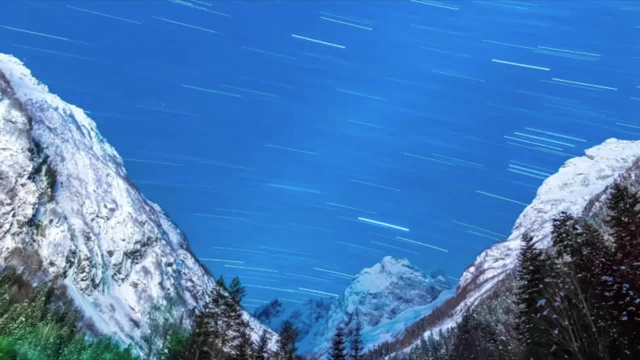 And I love giving these to my students because they're like how are we supposed to pick this out? But if you look carefully you can just see kind of make those connections with the pattern you already know. So here is where Orion is. You have the belt stars of Orion, You have Canis Minor. 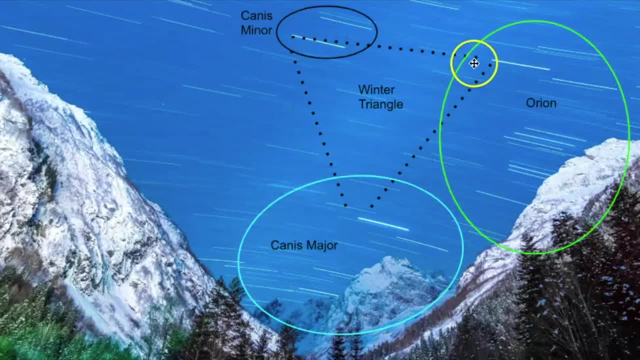 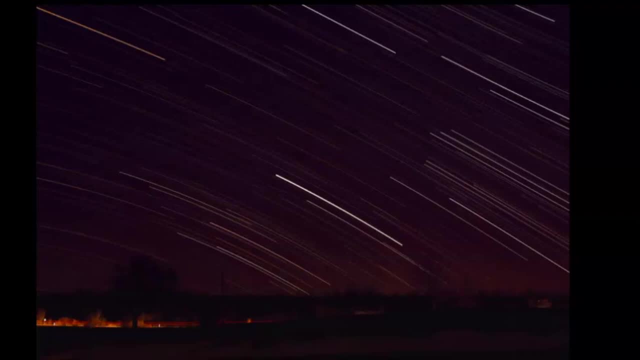 right here, Here's Canis Major, And then right here is where you would connect the winter triangle. Let's get one more shot here. Are you able to figure out where Orion is? Look for the belt stars. That's the key to finding this constellation, And then can you find the 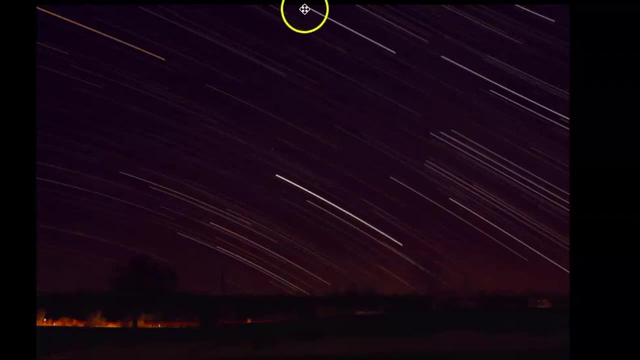 winter triangle. So here's the belt stars and then that's where the winter triangle would be. So this is like the ultimate test if you really really know your constellations is to use star trail pictures, And I think Orion is really the best one to do this with, because the belt stars 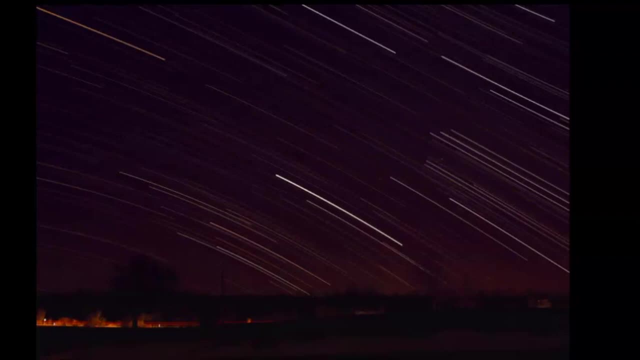 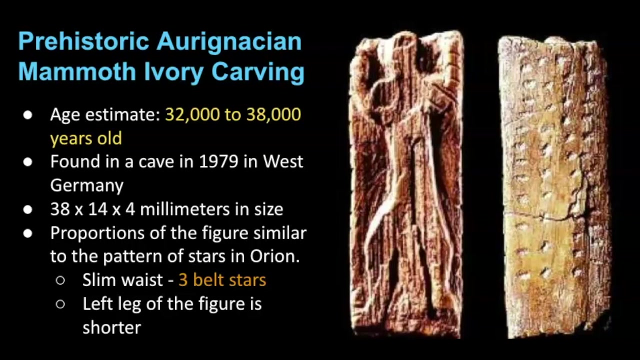 make these three long star trail pictures. Let's review some of the ancient mythologies that are associated with it. So first, the earliest known records we have of any constellation is that of Orion, And here you can see the prehistoric Aurignacian mammoth ivory carving that was found. 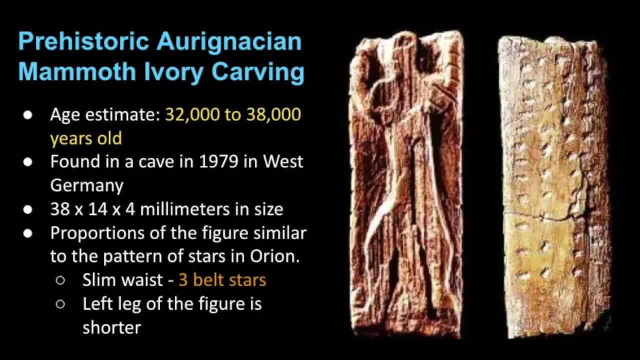 in a cave in 1979 in West Germany. Its age estimate is between 32,000 to 38,000 years old and it's pretty small in size, But its proportions of the figure are very similar to that of Orion. It has a very 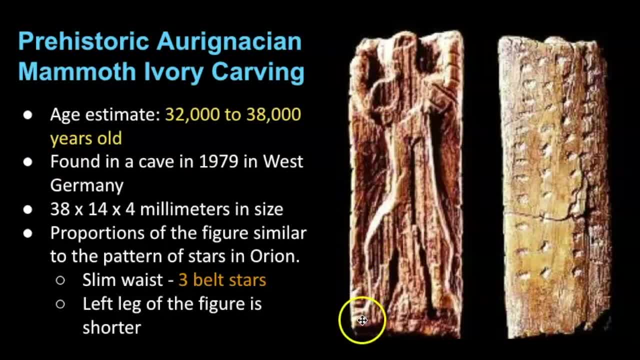 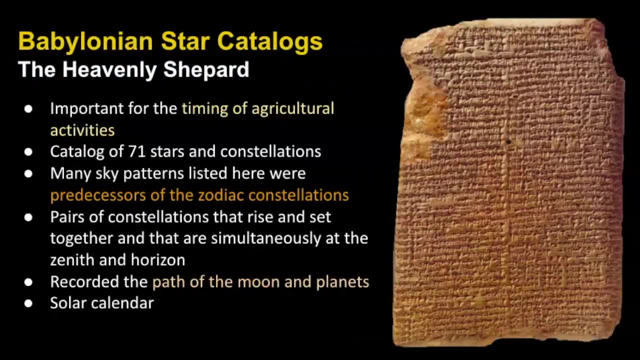 slim waist, just like the belt stars. And then here you can see, the left leg is shorter and that is very similar to that of Orion. After that we find record of Orion in the Babylonian star catalogs, and Orion was represented as the heavenly shepherd. The Babylonian star catalogs. 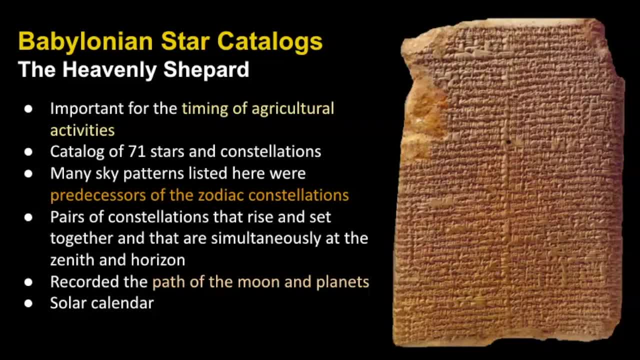 are really important for the recording and timing of agricultural activities. It also recorded the path of the moon, the planets. it had a solar calendar and it also recorded the path of the moon, the planets, and it also recorded the path of the. 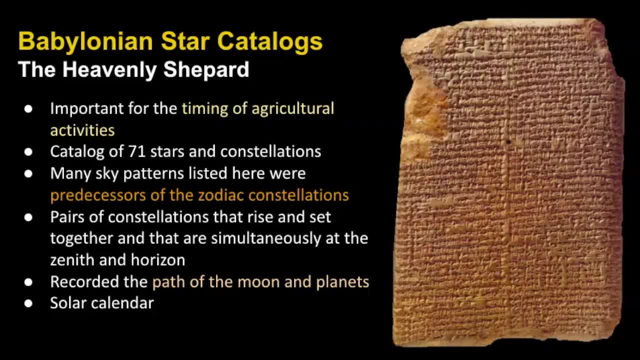 moon, the planets, and it also recorded the path of the moon, the planets, and it really, really was important for us to understand how the heavens move. so these agricultural activities could be timed. And many of these constellations on the Babylonian star catalogs were predecessors of the 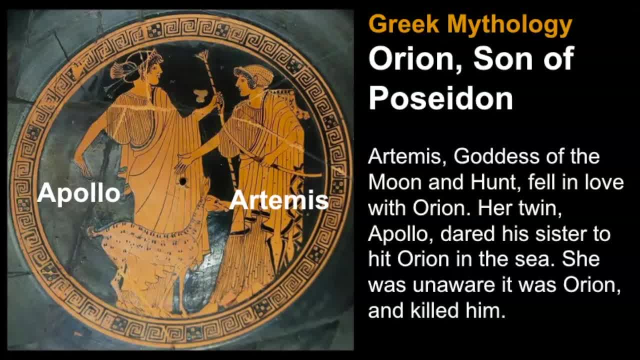 zodiac constellations. Next we'll jump to Greek mythology, which Orion was represented as the son of Poseidon And Artemis. one of the stories I discovered of Orion, and keep in mind there are many stories of Orion And Artemis- one of the stories I discovered of Orion And Artemis. one of 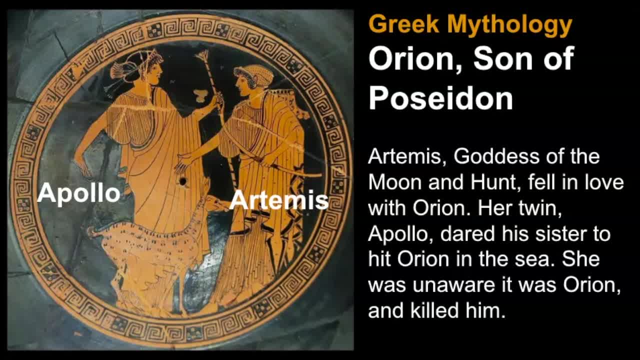 Artemis, the god of the moon and the hunt, fell in love with Orion, but her twin, Apollo, dared his sister to hit Orion in the sea with her arrow, But she was unaware that this was Orion and it unfortunately killed him. 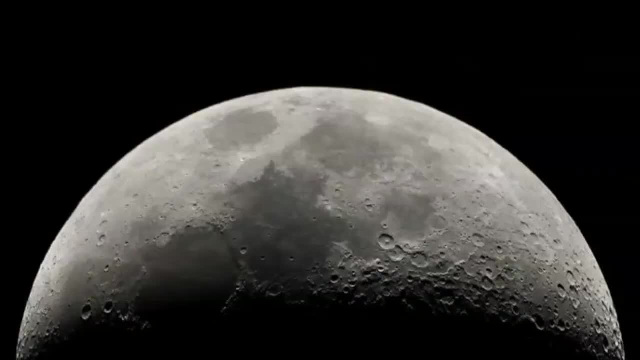 When his body washed ashore, she realized what she had done and in her grief, she placed his body in the sky along with his hunting dogs. It is said that that is why the moon is cold and lifeless, because Artemis lost the love of her life and was inconsolable. 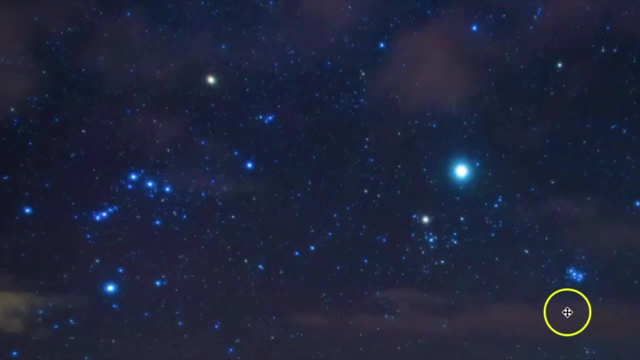 Orion, however, quickly recovered in the sky as he chased the Pleiades, which were the seven beautiful nymphs in the constellation of Taurus. In one myth that I found, Orion right here fell in love with the Pleiades, the seven sisters. 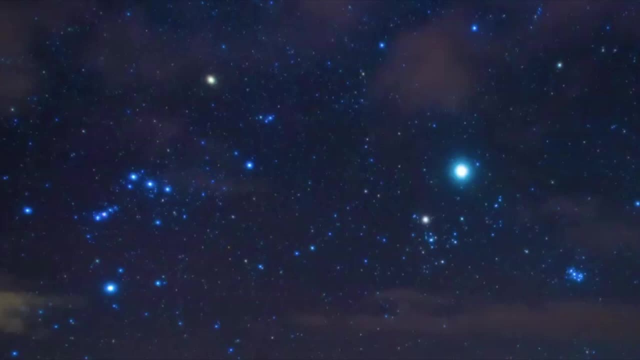 And the seven sisters were the daughters of Atlas and Pleiades. He started pursuing them, so Zeus scooped them up, placed them in the sky, and the Pleiades are representative of these seven sisters, And it is said that Orion is still chasing them in the sky. 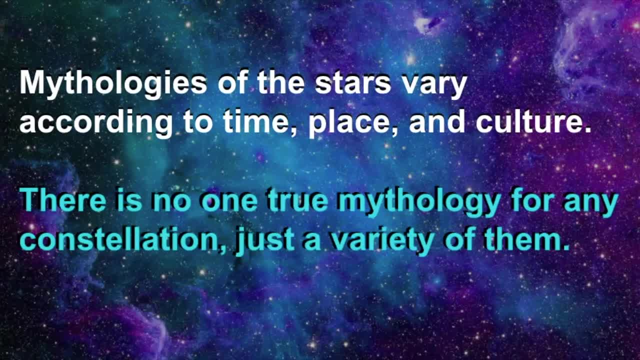 But again, these are only a small portion of the mythological tales of Orion. Remember that the mythologies of the stars vary according to time, place and culture and there is no one true mythology for any constellation, just a variety of them.